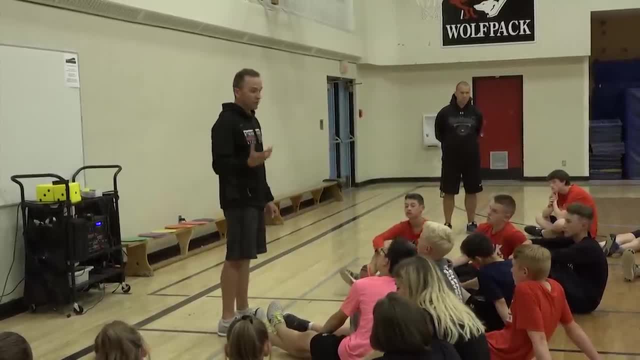 least six groups in the center circle. We're going to have eight groups in the center circle. We're going to have eight groups in the center circle. We're going to have eight groups in the center circle. We're going to have at least eight people in the center doing an exercise, If there's anyone that. 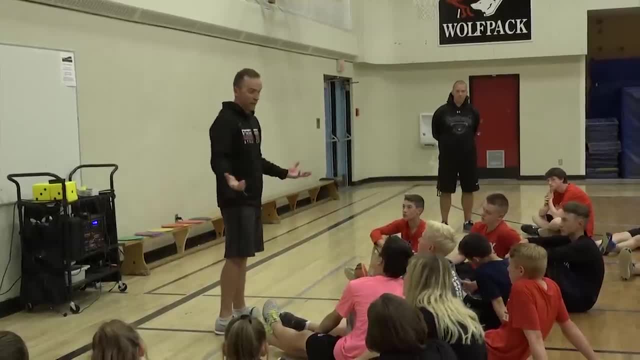 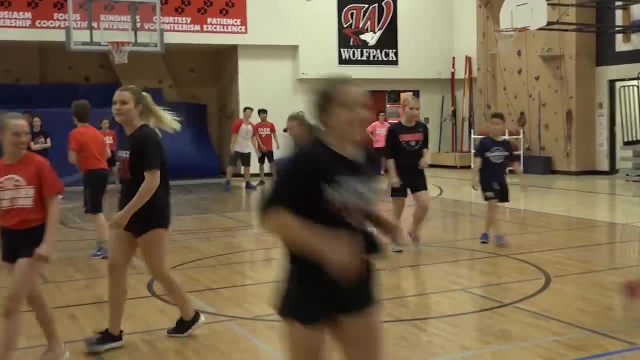 wants to come out and join one of their group members and be a good teammate and do the exercise with them, that's fine. And you complete that exercise and then you just go back to your groups afterwards and we'll decide which side's going to start us off when the music goes. 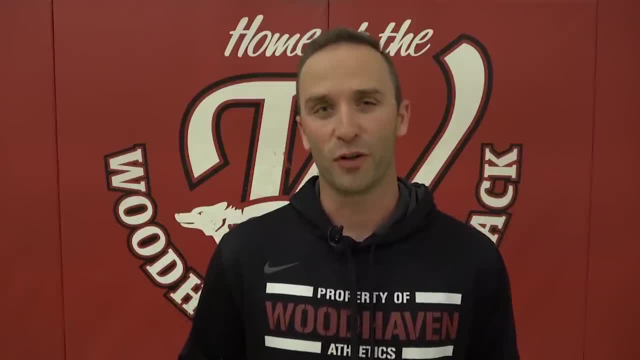 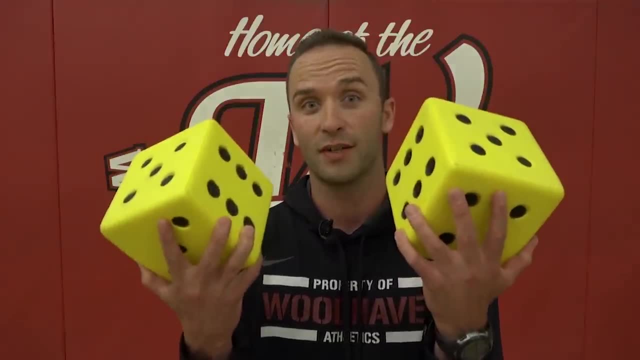 In reality, you could play snake pit without any equipment at all, but it's much more enjoyable and a lot easier to do if you do have a stereo and some music that you can play. We also use two foam dice that we use to determine the number of repetitions for each exercise. this 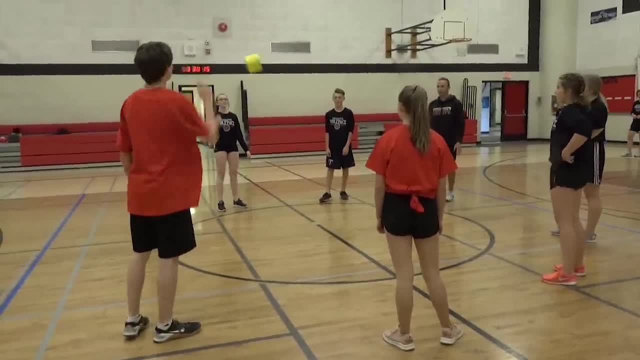 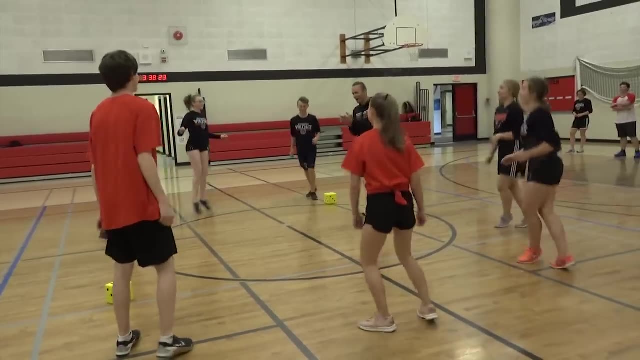 students will do All right. so we're multiplying this. Let's see it. We're going crisscross jumps 36. crisscross jumps- Awesome. Let's get started With younger groups. it's usually a lot easier. 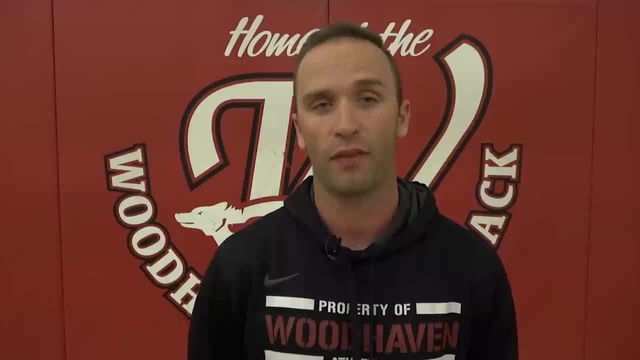 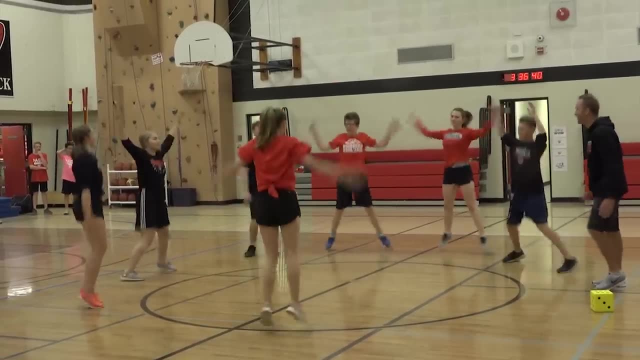 more effective if the teachers select the exercises that they're going to be doing That way. if they need to demonstrate the proper technique or proper form, they can do so. We try to start with some basic ones, such as jumping jacks or crisscross jumps. 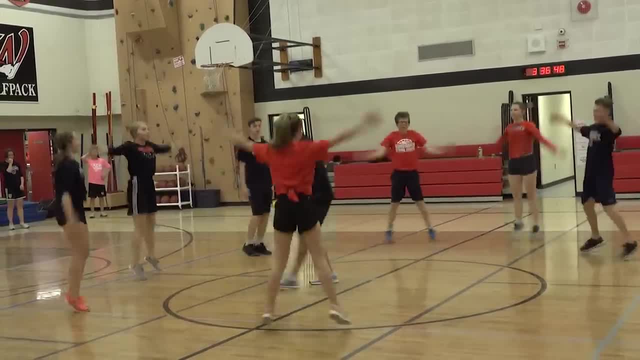 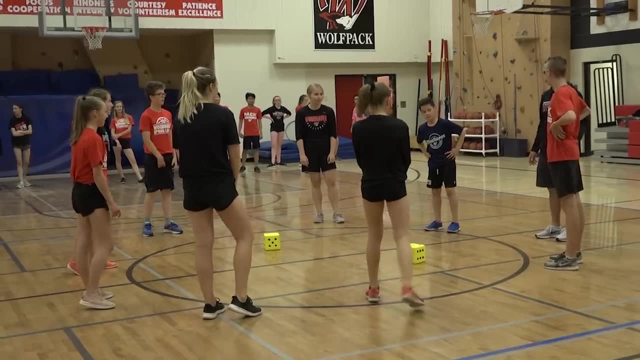 things that the students have done before. nothing we really have to demonstrate With the older grades- sometimes they're grade eight, grade nine students. we give them the opportunity to choose their own exercises. We can incorporate some more difficult ones, such as push-ups or burpees or even squats, And then, if we need to slow things down and 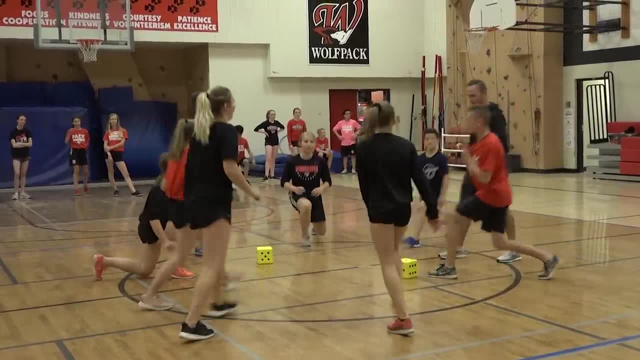 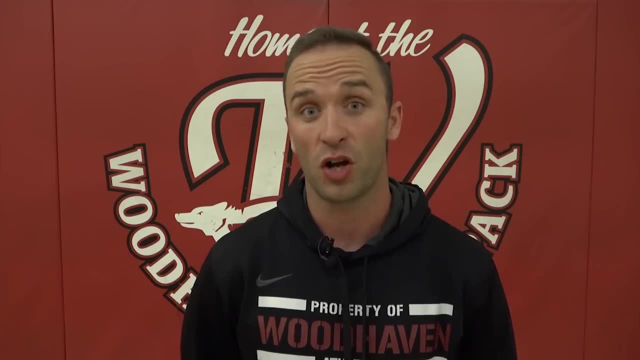 demonstrate some things, maybe some core exercises like mountain climbers, things like that. Some of the different movement patterns that you can do just while going from one of the gym to the other could be as simple, starting with a jog, but then as simple as maybe a. 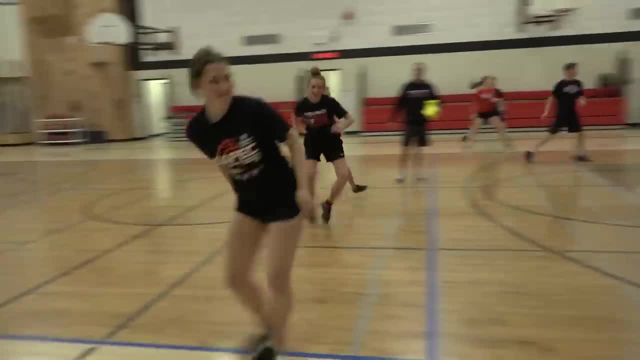 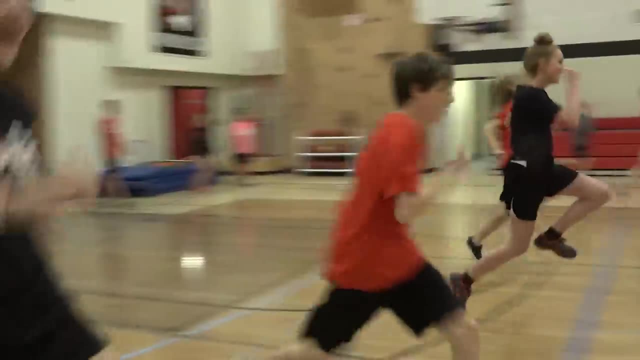 lateral shuffles, meaning they're all facing one side or one wall in the gym and just staying nice and low and shuffling laterally all the way there. It could be as simple as skipping right, Or one foot hopping, two foot hopping, anything that just gets them. 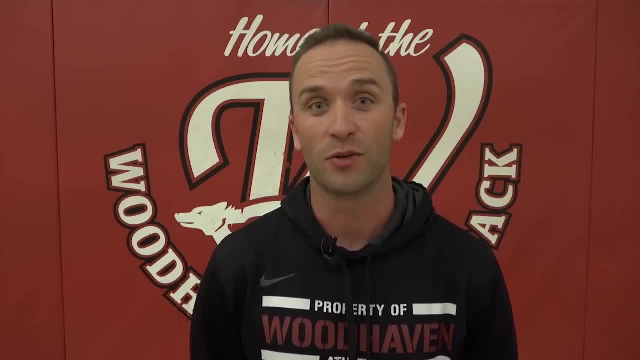 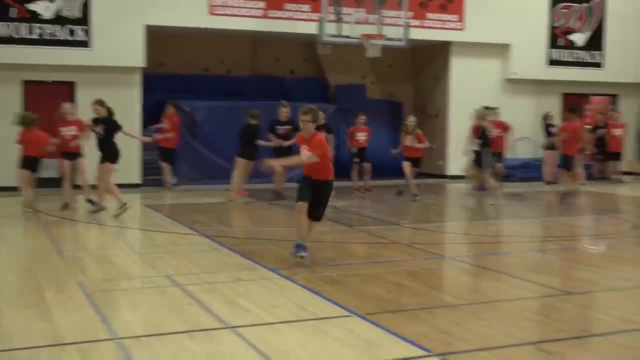 moving in a little bit differently. Snake pit is a great activity to do as a warmup. It gives the students an opportunity to kind of build up their cardiovascular endurance as well as work on muscular strength and endurance. Sometimes it's just a great way for the students. 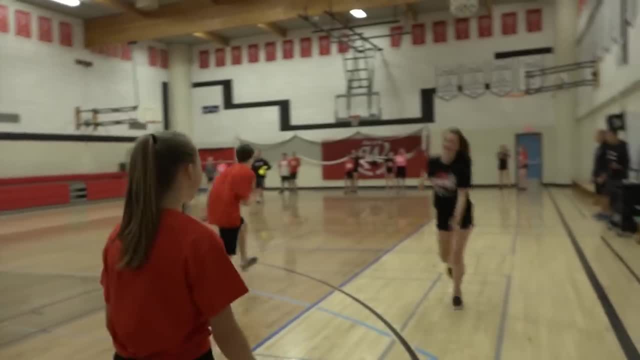 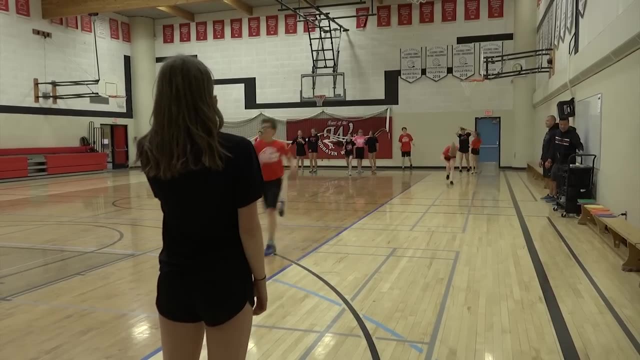 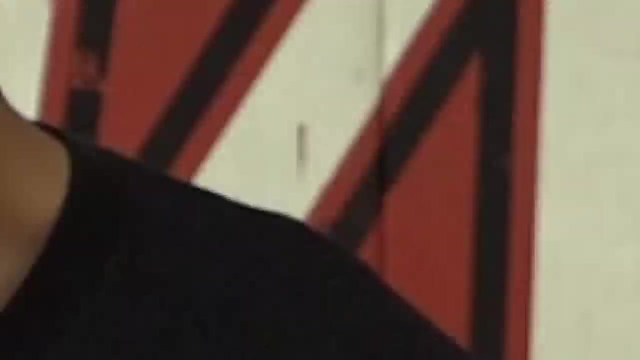 to run and get moving and burn off a little bit of energy. Also, if you get an opportunity to incorporate different movement patterns rather than just jogging, then it helps students focus on their physical literary skills as well. The next game we're going to show you is called Dice. Tag. This is a great game for the elementary grades. It can probably start in grade one and work your way up to grade 12.. The amount of kids I'm going to play this with is probably 20 and up, as it depends on the size of your gym. 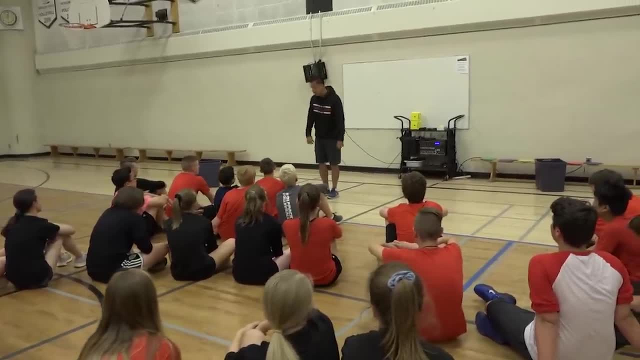 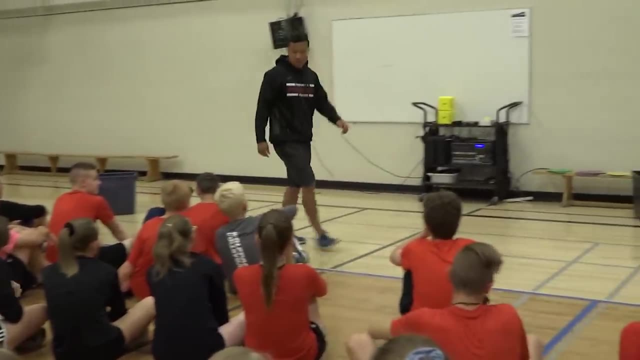 The object of this game is to not get tagged. We have a team over here. You must have one foot on the grade line. You line up across here The other team. they line up on this grade line and you're across this line here. What we're going to do, we're going to roll two dice. 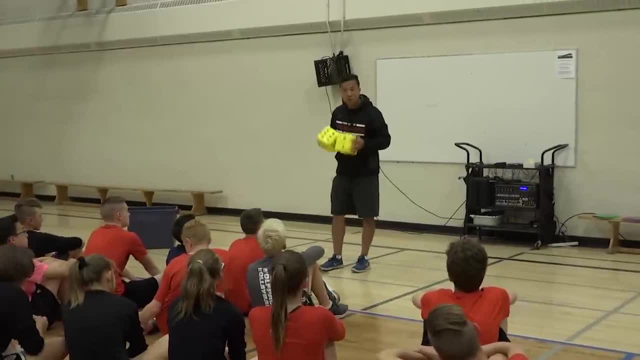 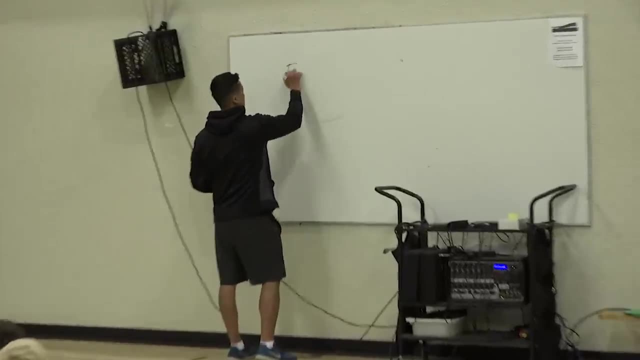 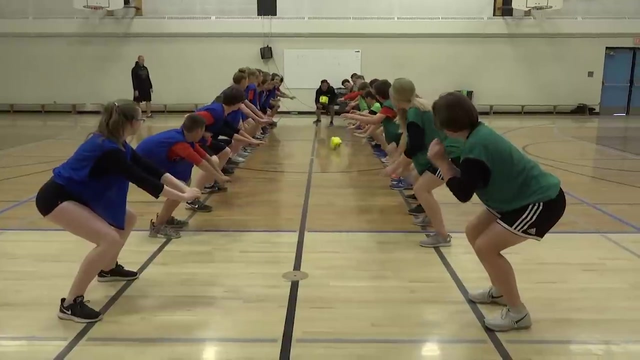 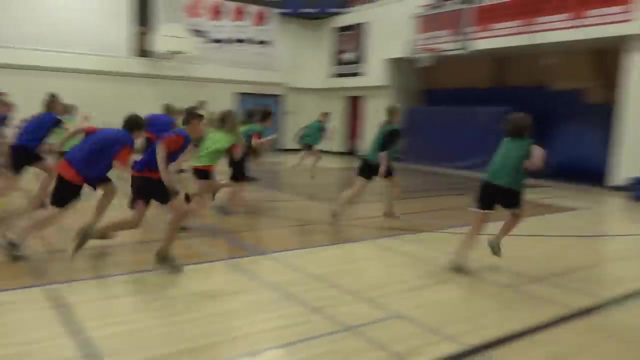 and we're going to add subtract maybe, or multiply. Now this side over here will be even, Okay, and this side over here will be odd. So if we roll an odd number like two plus one, the odd team, you have to sprint back and pass that blue line without getting tagged by the even. 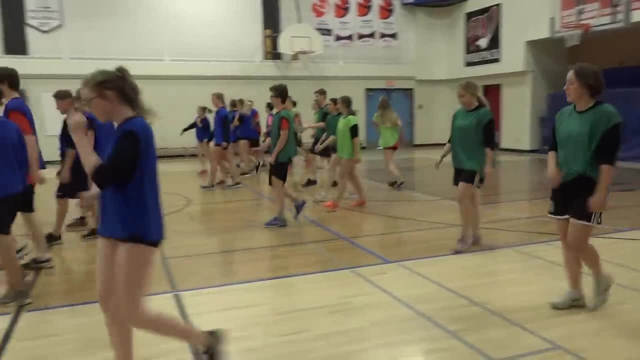 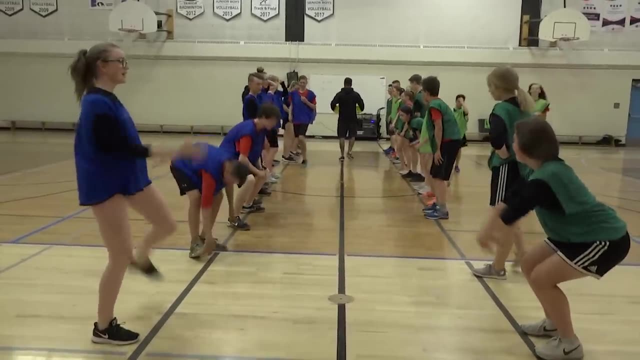 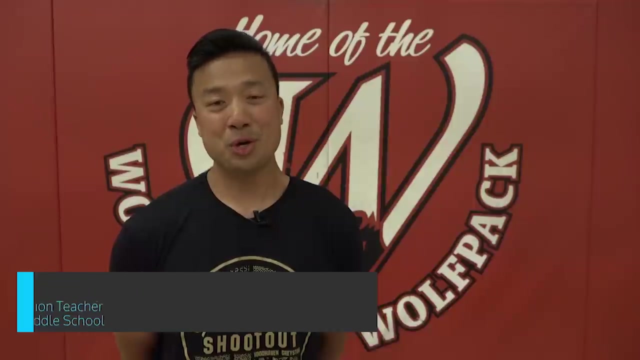 team. If you get tagged, you would run back and you would come to the teacher and do five jumping jacks or an exercise of the teacher's choice and rejoin the game. If, for instance, you were to run the opposite way and it wasn't your number, you would also have to go and do. 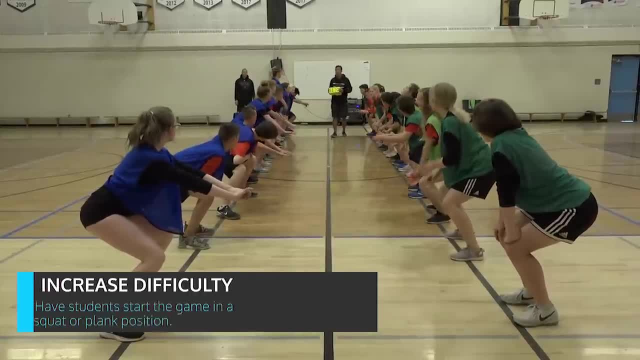 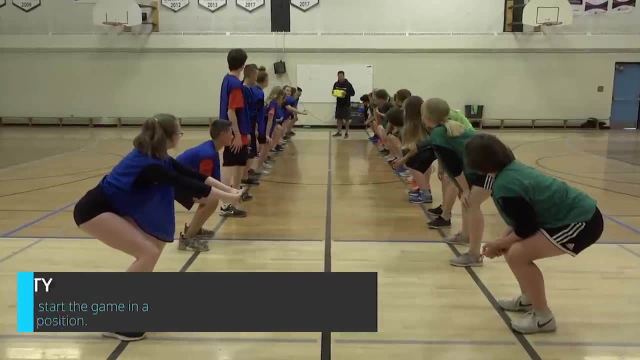 an exercise of the teacher's choice. Let's, let's subtract, So it's always bigger number subtracted by the smaller number and zero will be even. I'm gonna throw them right now. Put that once. mess you guys up here. 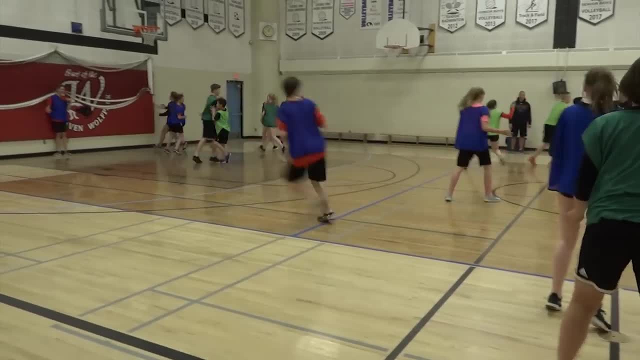 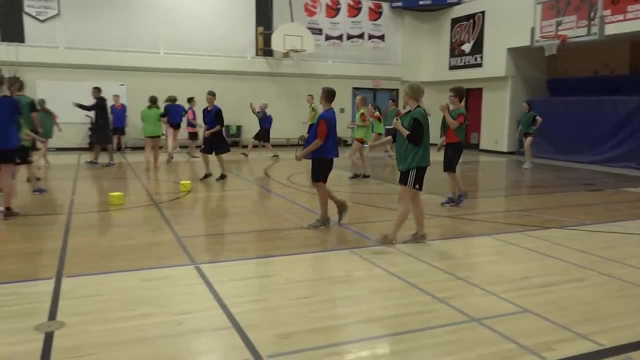 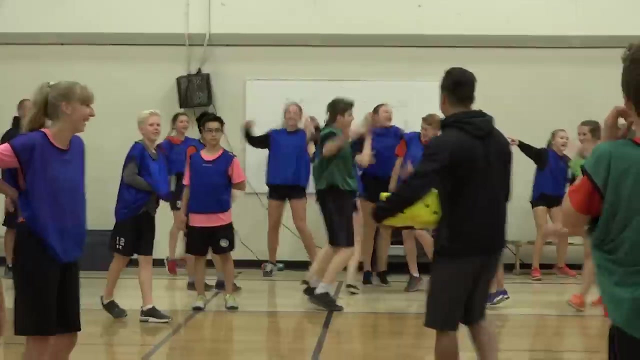 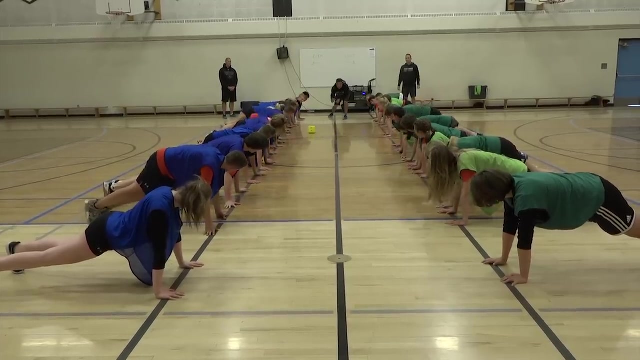 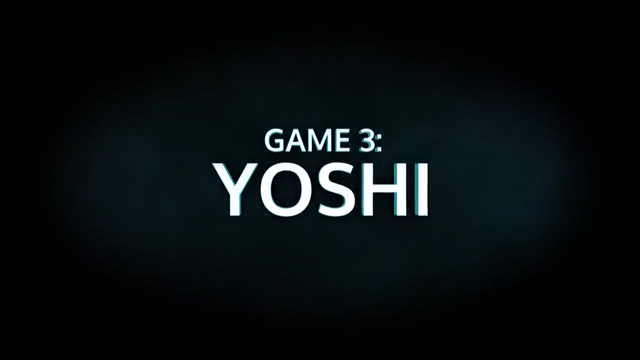 Oh no, That's odd. You guys all have come over here. You guys are all. I'm smart, I'm smart. There is really no end to this game. It's a great game for warm-up and it's also a good game to teach a little bit of math skills and get a lot of activity involved. 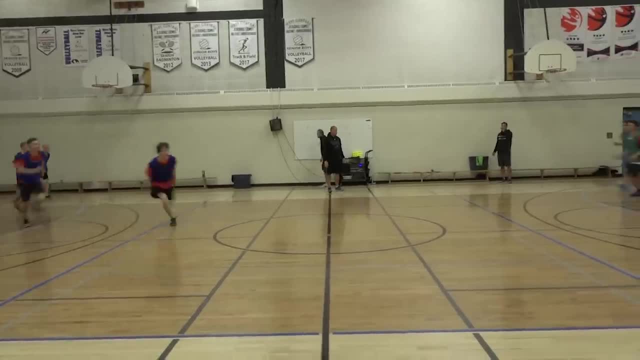 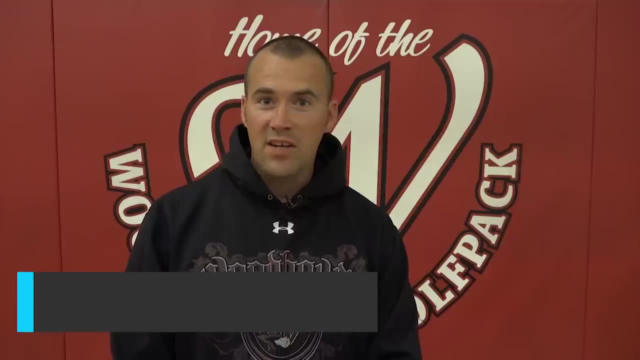 The next game we'll be playing is called Yoshi, So you can play this game with 20 to 80 kids, grades 5 and up. To play this game, you'll need a large area of space. If it's outside, you can have some cones, but as long as there's court lines and a gym floor. So the game of 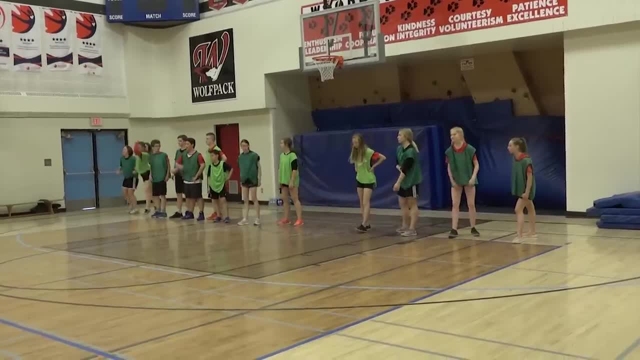 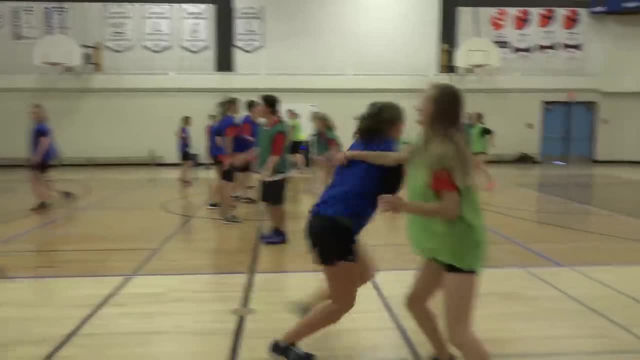 Yoshi is played with two teams on two different sides of the court. Your ultimate goal is to get your entire team over to the other side past the safe line. If you cross the center line and you're tagged, you need to sit down where you got tagged. You can, however, 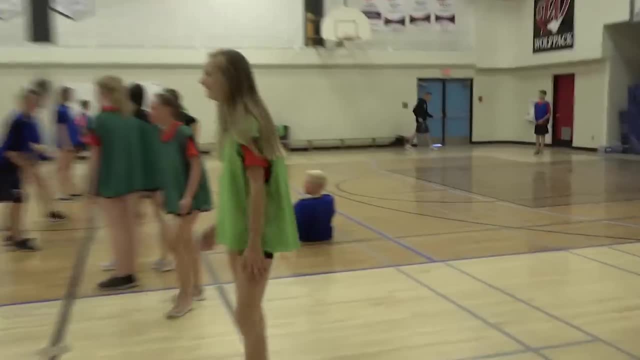 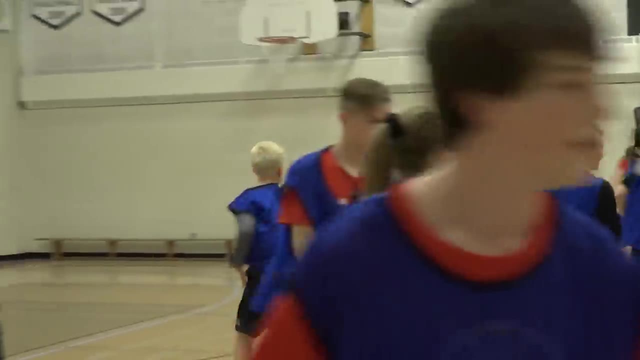 be saved by one of your teammates, either from your side or someone who leaves the safe zone to save you. But when you're saved, you need to go back to your side before you can go to the safe zone. When I yell the word Yoshi, no more tagging, at that point Everybody 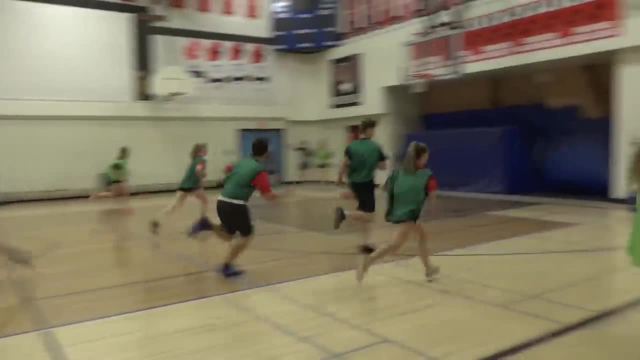 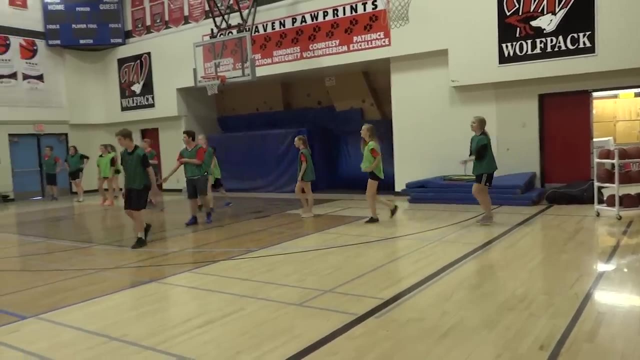 sprints to the safe zone. If you're already tagged and Yoshi has been called, you need to be saved by another teammate before you can get to the safe zone, before your team can win, One of your teammates will have to come grab you, bring you back to your center line and then you can go to the safe. 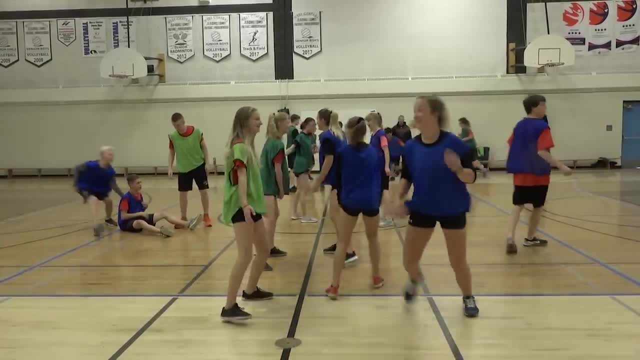 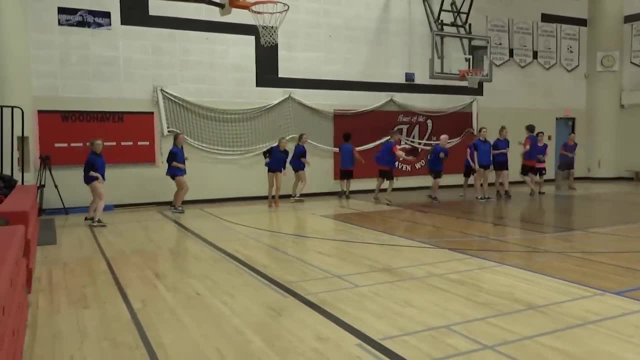 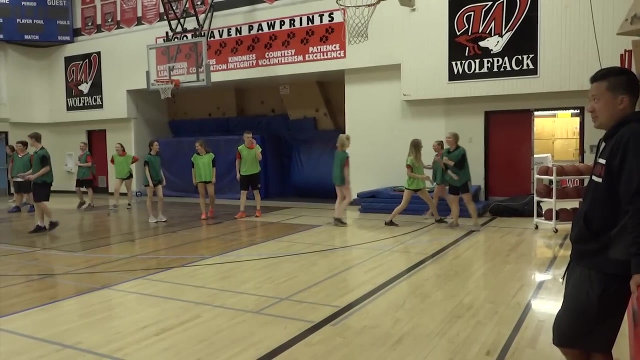 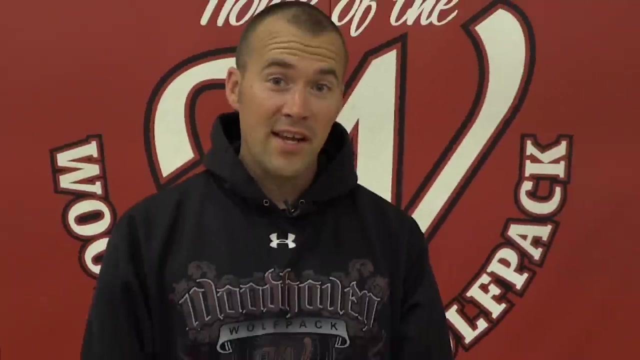 zone. The team that gets all their players saved and over the safe line first is the winner. Yoshi The blue is our winners that time. The next game we're going to show you is called Aladdin Slide. This game is best suited for 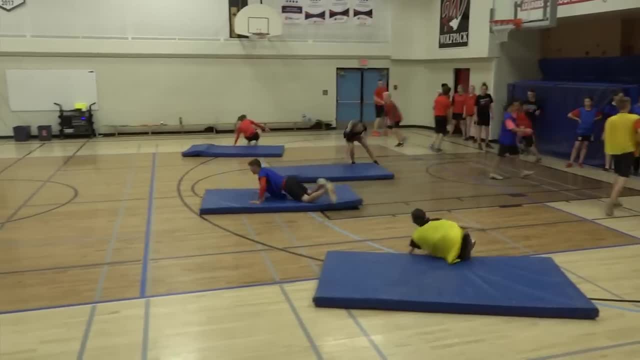 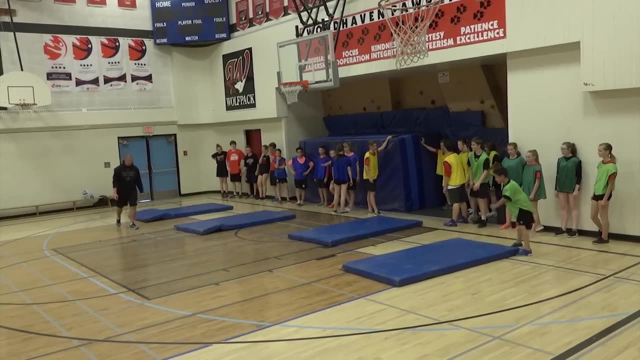 students in grade 5 and up, and you can play upwards of 20 to 50 students. To play this game, you're going to need some mats, usually about the size of the students, and they're going to be decently thick so that way students can jump on them, And you'll need some pennies. 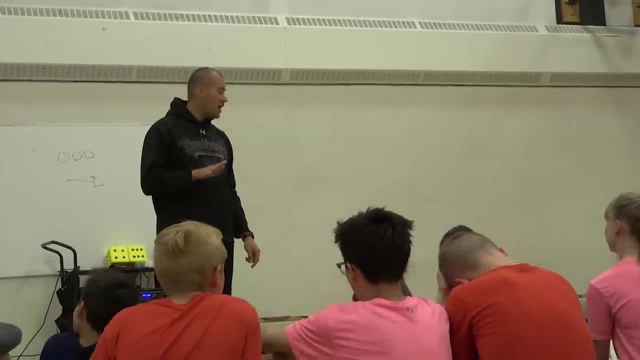 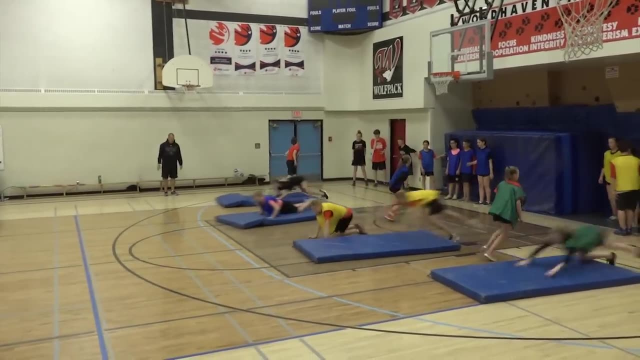 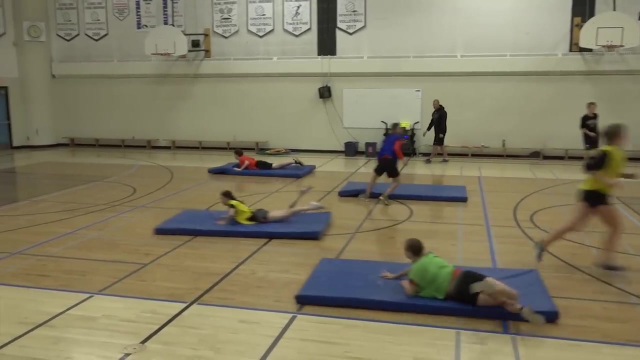 to divide up into different teams. Your objective is to dive on your belly and slide that mat. So after one person jumps on it and you dive when one person rolls off of it, the next person in your team line will run diving on the mat. The goal is to slide the mat all the way down to touch that. 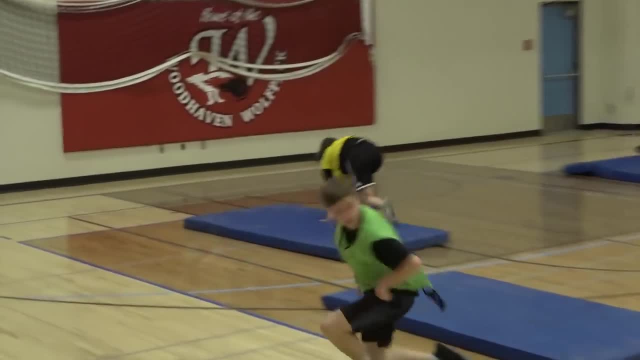 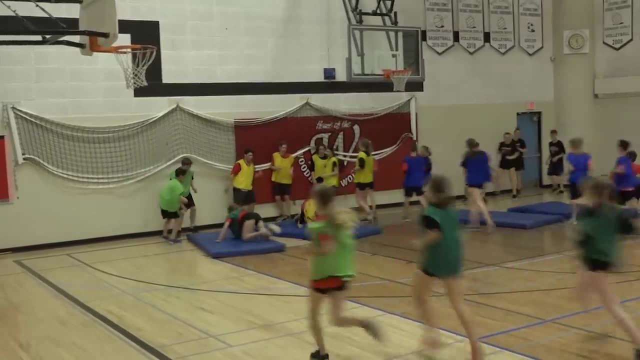 blue line. Once that happens, the rest of your team runs behind you to restart over there, trying to go all the way back. So you're going to get that mat to go from the starting point all the way to the blue line and then all the way back in a relay style race. 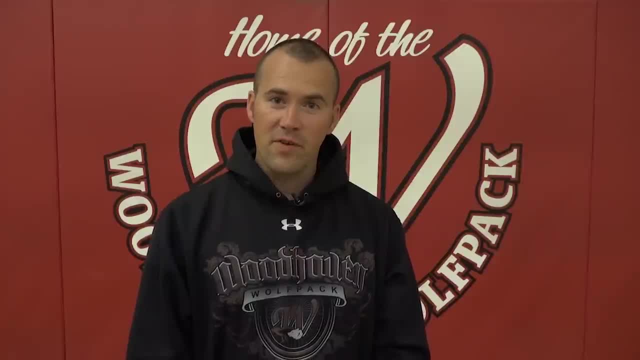 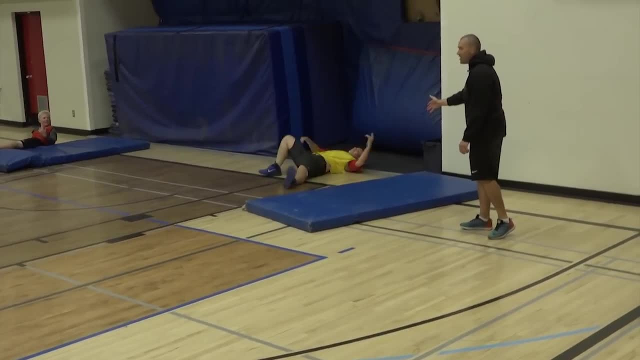 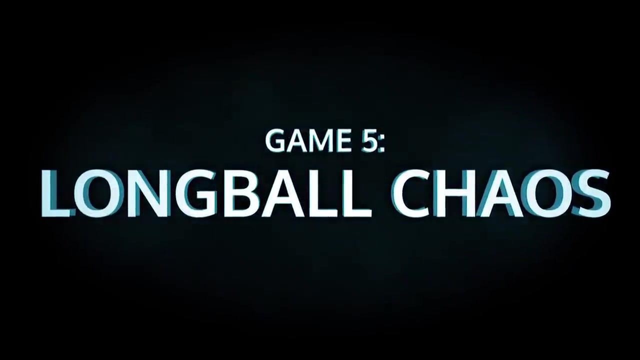 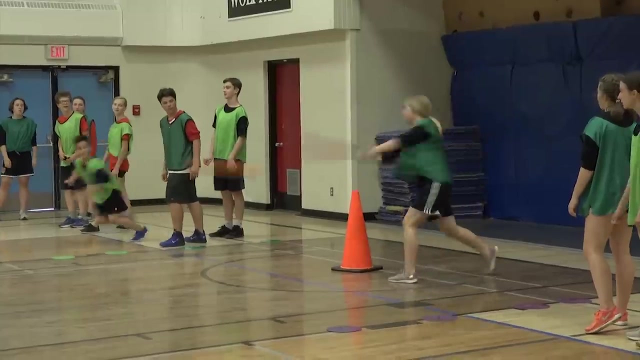 The team that gets to the starting point first after the turn around is the winner. Yellow did it, Yellow did it. Yellow did it Yellow with the victory. So the next game we're going to play is called Long Ball Chaos. Ideally, this game is best. 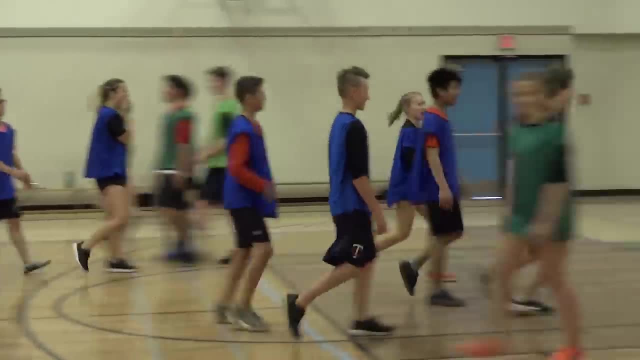 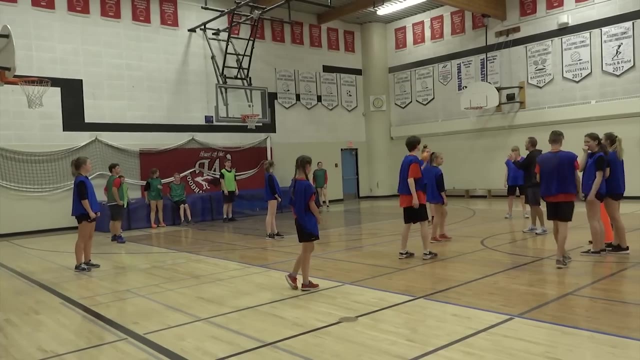 with 25 to 50 students, When you're playing with larger groups- even sometimes with 60 to 80, you just need to be a little bit more creative in how you split the students up into teams. Sometimes, instead of doing two teams, you could have three teams, with one team sitting out for a few minutes. 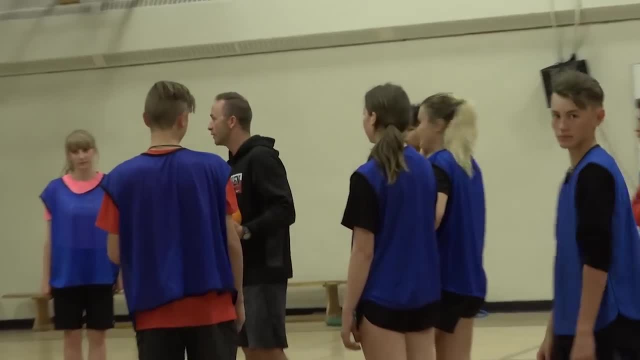 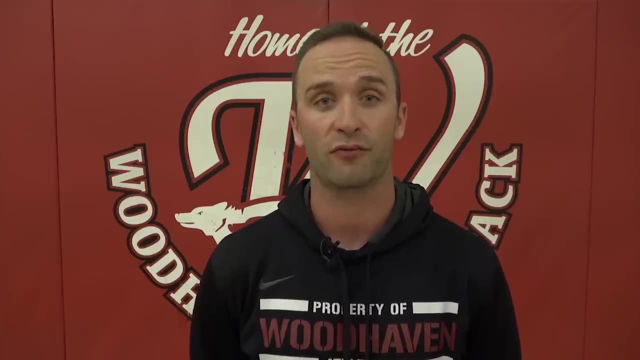 and watching and then rotating, But 25 to 50 is kind of that ideal number. We do this activity with all of our students here, grades five to nine, And once again you could probably adapt this for any of the younger grades and older grades in high school as well. 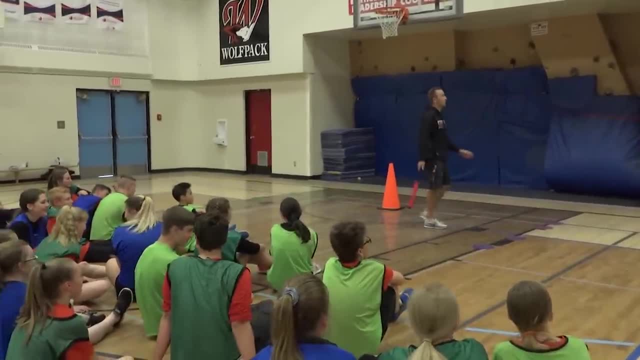 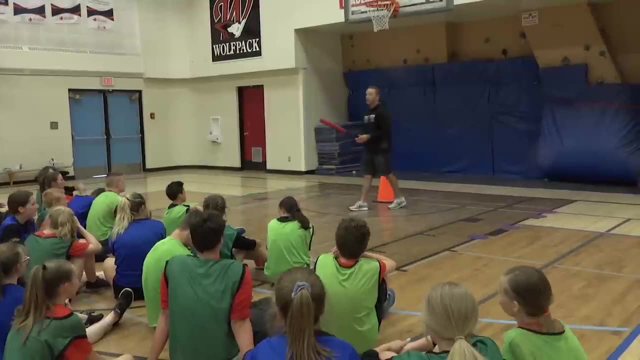 So for this activity, the equipment you will need is a foam baseball bat, one foam dodgeball bat, two large pylons, and it'd be great if you had at least one high jump mat. Two would be even better to use as safe zones If you don't have access to those that's. 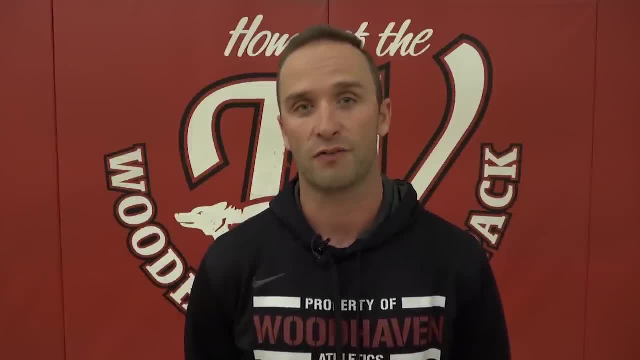 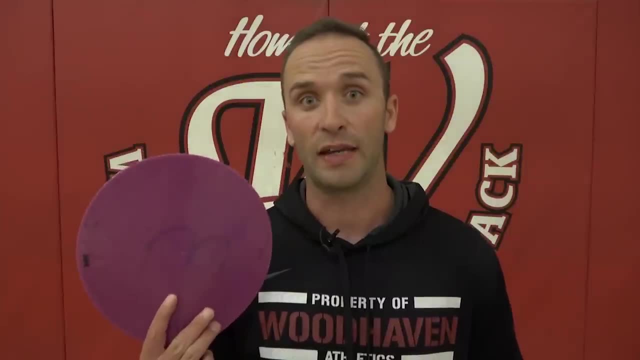 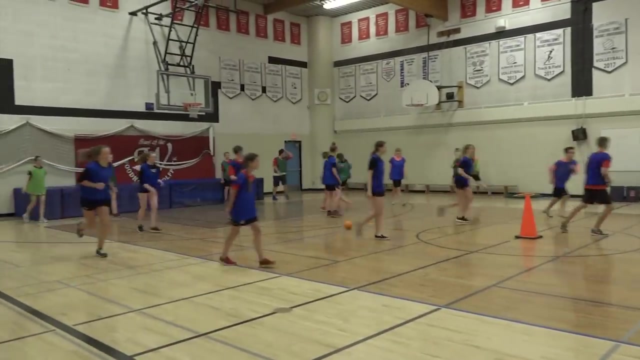 okay, You can just identify certain lines on the gym floor to create safe zones. Also, we like to use either small pylons or poly spots such as these just to identify a hitting zone that only the batter will be standing in. So Long, Ball Chaos is a two-team game. There's basically one team on defense and one team. 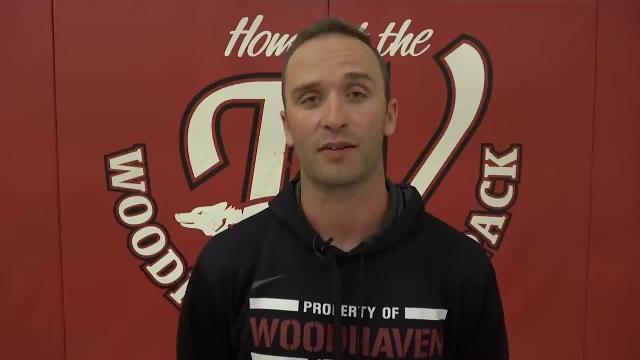 on offense. I'll start with the defensive team and kind of their objectives. They're basically trying to earn outs or get the offensive team out, similar to they do in baseball, And in order to do that, they can either catch the ball once it's been hit. they need to catch it. 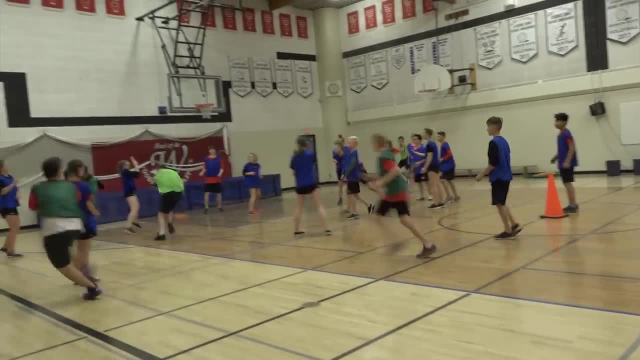 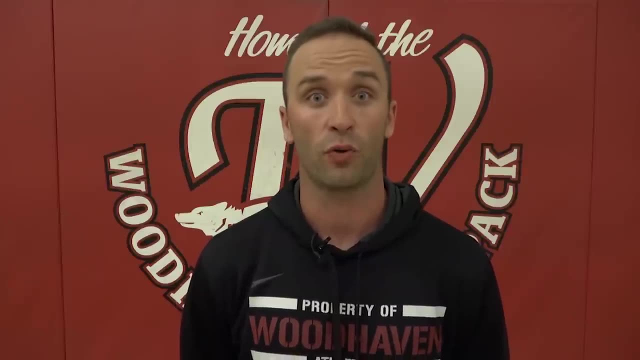 in the air before it hits the ground, or they can throw the ball and hit any of the runners before they get to a safe zone. Now in our gym we like to say that the ball is live off of the roof or the walls, So that 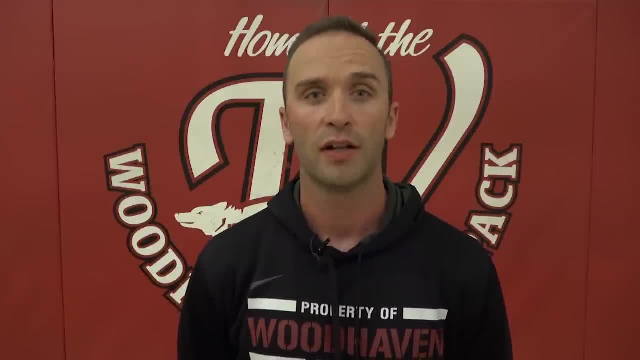 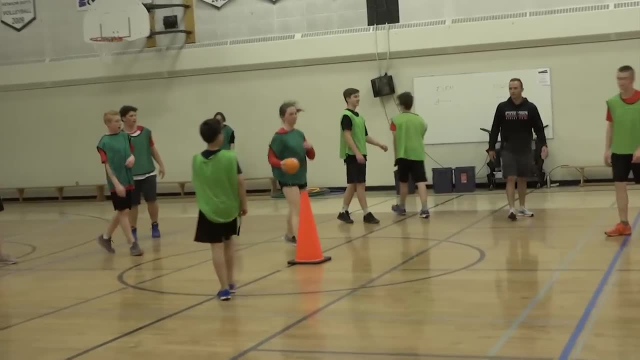 means that if the ball is hit off the roof or the walls and caught in the air, then it's still considered an out. If the defensive team is unable to get any of the offensive players out, they can simply take the dodgeball, go touch the cone that's in the center of the gym and that just basically. 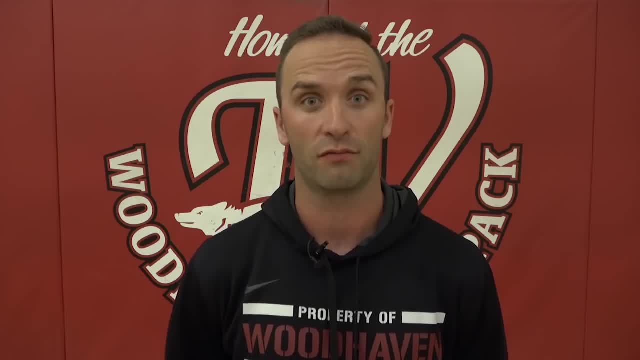 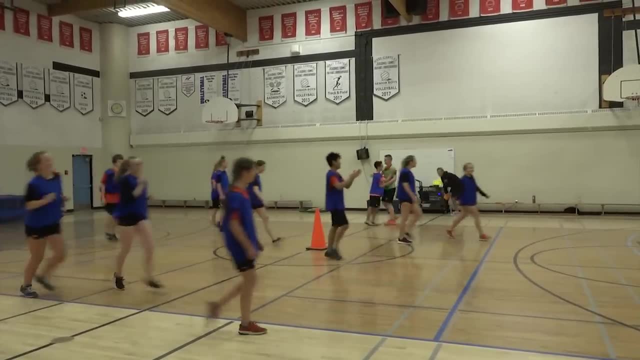 signifies the end of that round and the offensive team can no longer run. If a player on the offensive team gets hit by the ball, or if the ball is caught in the air and the defensive team earns an out, then basically the offensive and the defensive. 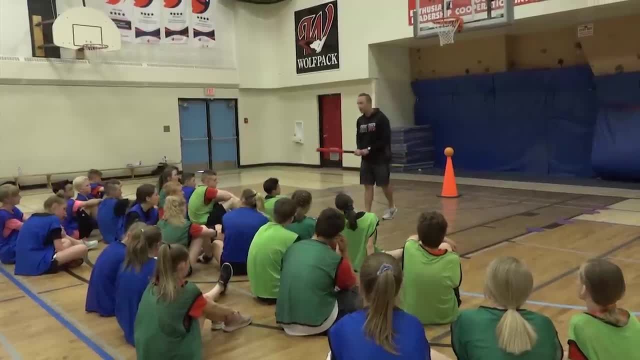 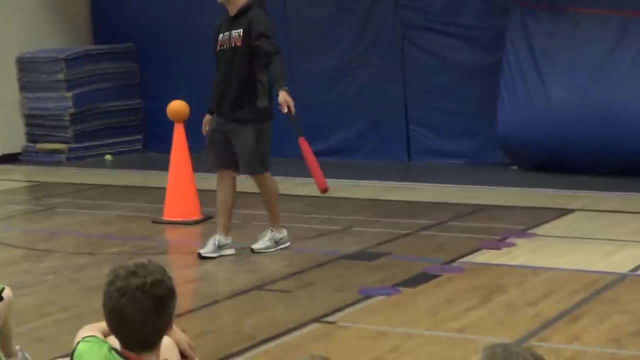 teams will switch spots. Offense then, right, We do have a batter, like in baseball. You'll see here, right, that we've set up some poly spots. This is what we're going to call the hitting zone. Only the person that's batting can stand inside this zone, all right. 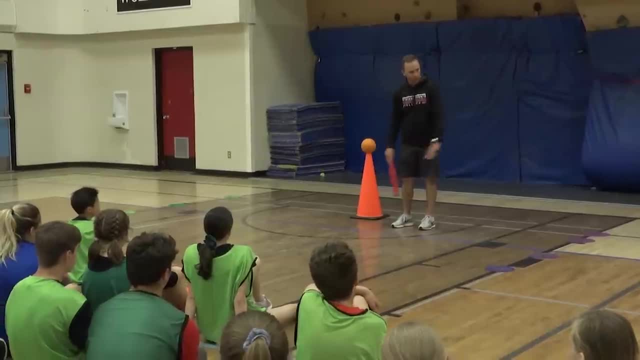 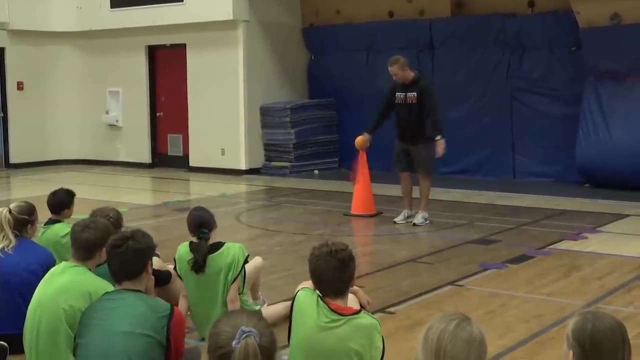 The rest of the players you're going to be just spread out, the rest of the offensive team spread out behind this blue line. all right, Because this blue line here, right, that indicates one of the safe zones. We have one safe zone here behind this blue line. 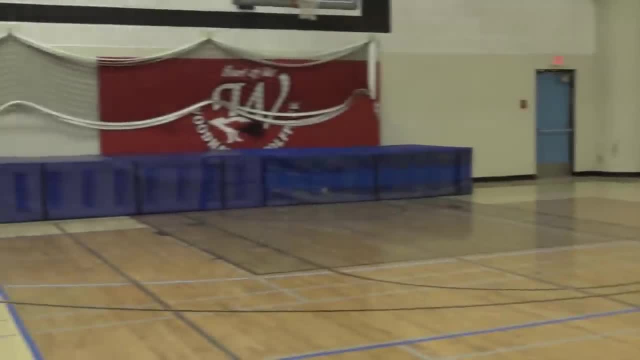 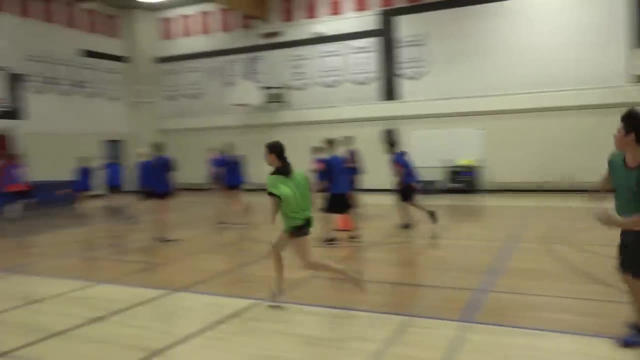 The other safe zone are the high jump mats there. okay, And don't worry, I'll show you on what those mean. all right, So each round starts, right. One person's up hits the ball. okay, Now the person who hits the ball. they have to run, just like in baseball, right? 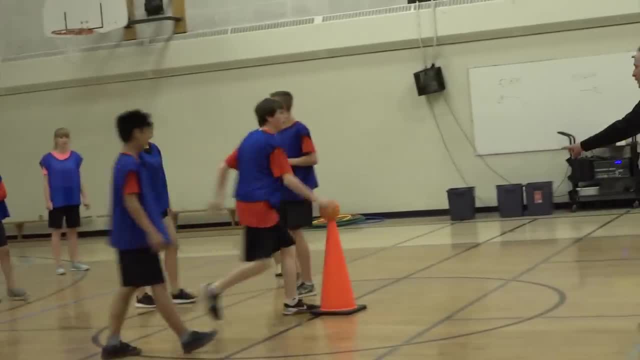 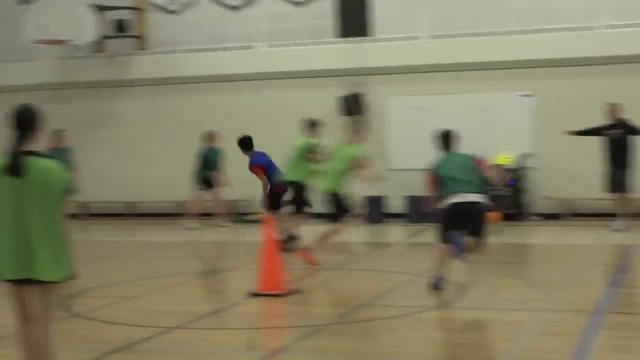 They have to try and get to that safe zone. all right, If they get all the way to the safe zone, they can choose. I can either try to come back to this safe zone here, which scores us a point, or they can stay there if they don't feel it's safe or they think. 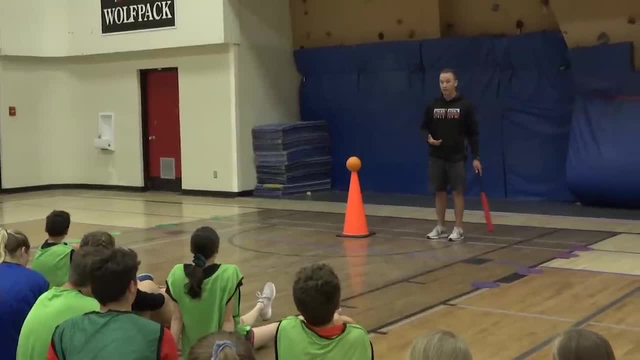 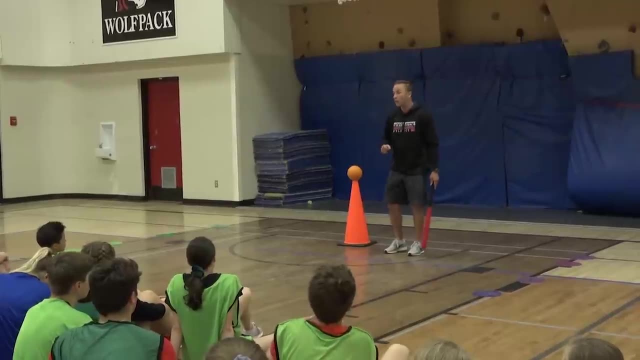 they might get hit. The way it's different than baseball, though, is that everyone else that's lined up here the offensive team. everyone here has the choice of who's going to run or not, So we might have one person running, just the person who hit, or we might. 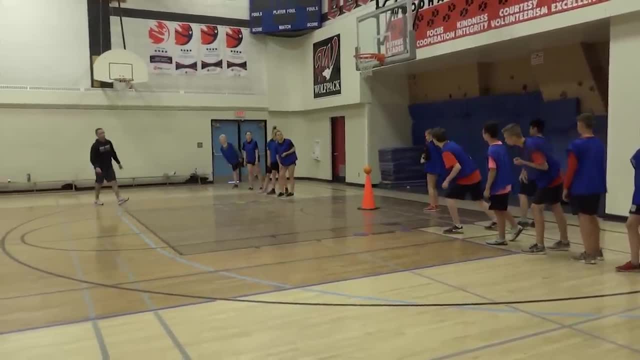 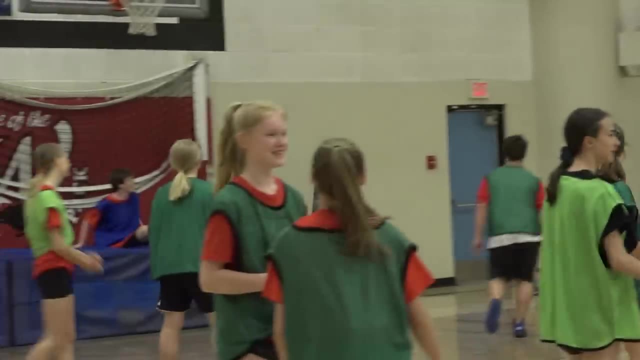 have all 18, 25 people on a team running at once trying to get to that safe zone. Every time an offensive player gets all the way to the far safe zone and back, that basically creates one point for their team And they can continue to do that as long as the play. 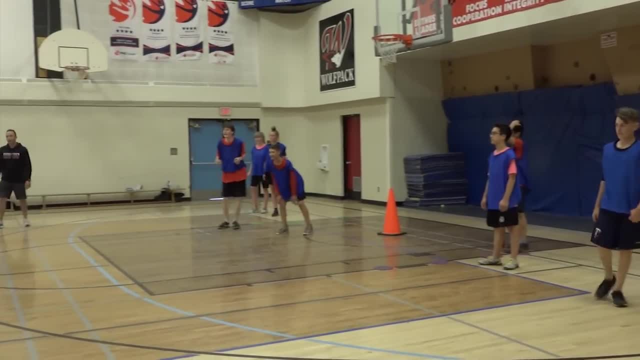 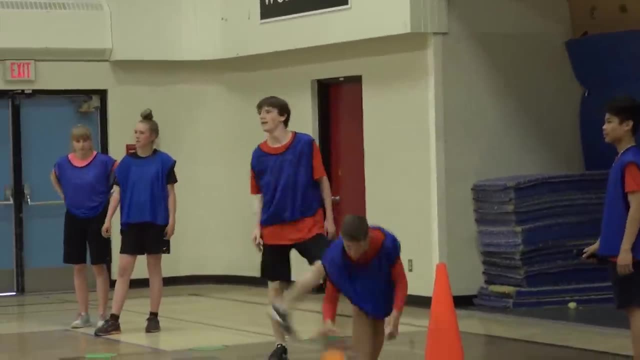 continues. That play continues until the defensive team hits them with the ball or the defensive team takes the dodgeball and touches the large pylon. Now, if you made it all the way to that safe zone and back, that means if you scored a. 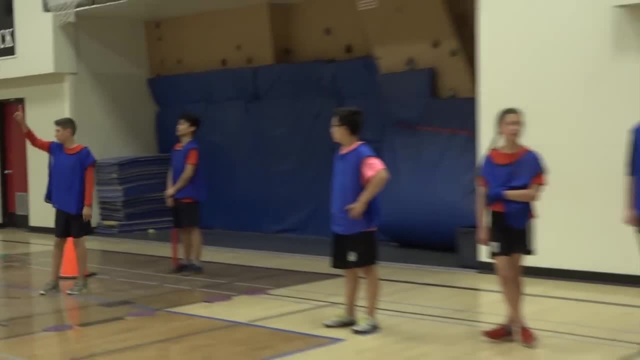 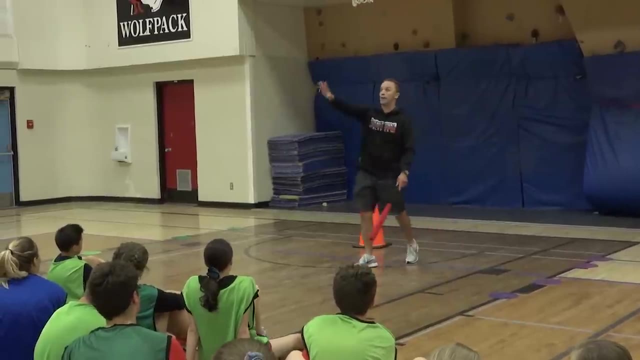 run, put your hand up, show me how many you scored. We got one, two, three. Anyone else over there? Okay, so now it's 3-0 for blue. Sounds simple, right, You just run there, touch that and come back. right. But it is tricky in the fact that you don't want to. 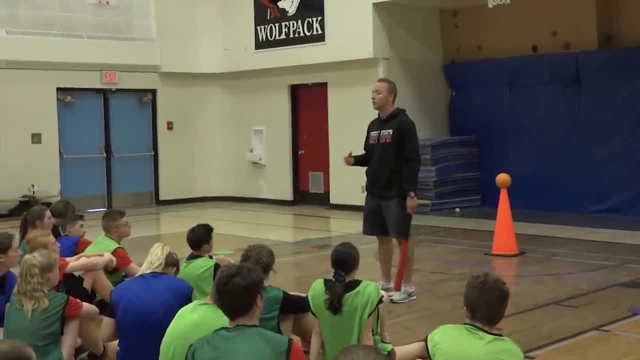 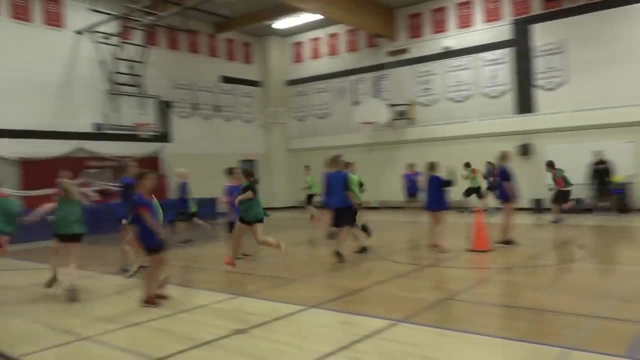 be too risky with your running right. You don't want to take too many chances because if, at any point that you're running trying to get to a safe zone or back to this safe zone, if you get hit with a ball, then none of the points count or none of the runs count. 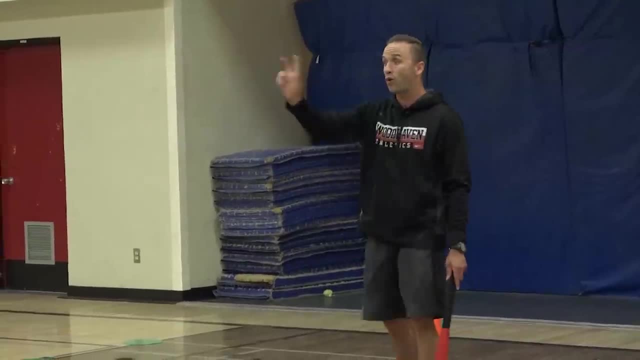 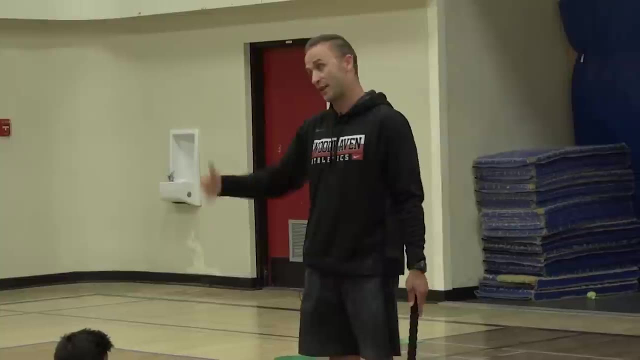 that anyone's earned that round right. So you might have 12, 15 people, get there and back and possibly score 12 or 15 points, but if someone gets hit with the ball that round it's an out and none of those points count. 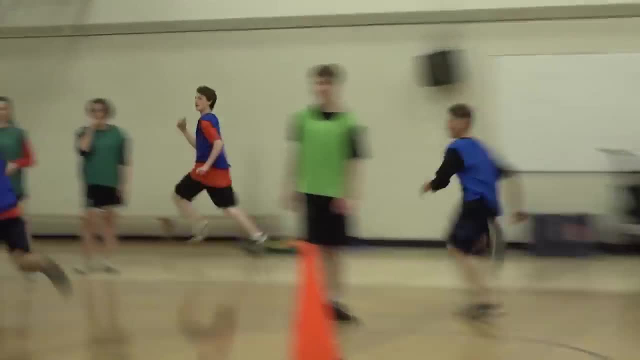 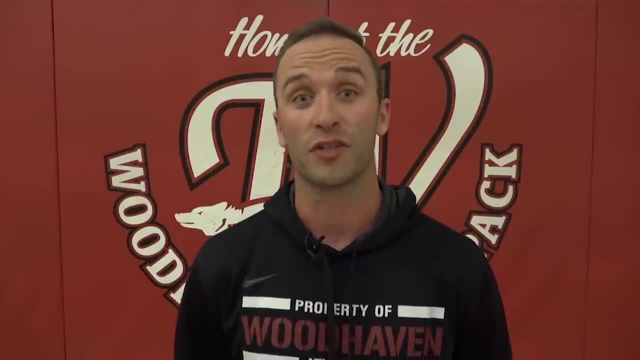 You know we play this game because it allows the students to focus on several different skills, such as batting, throwing, catching, but it also gives them an opportunity to communicate with their teammates. There's a level of kind of cooperation that they need to make sure they're working together. 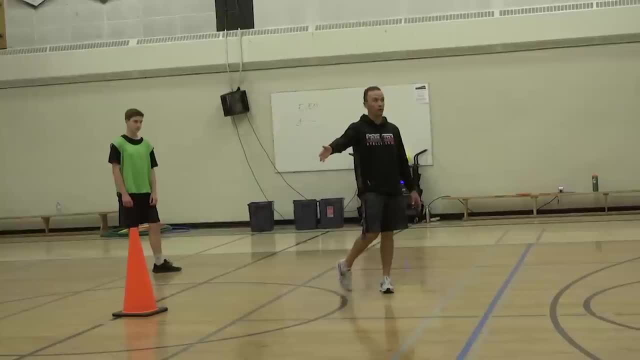 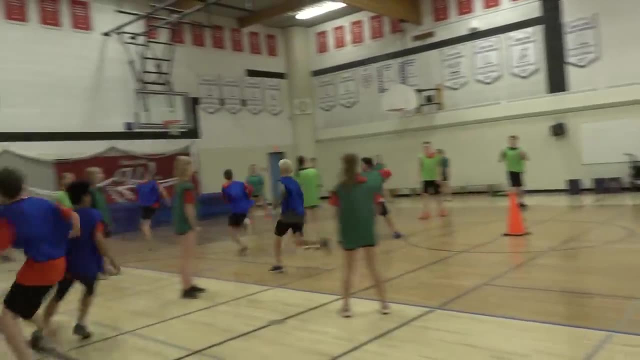 in order to decide when to stay and when to run and you know what? also because they seem to really enjoy it. They enjoy hitting that ball as hard as they can and some of them just love to run. so some of them will continue to run and try and score three or 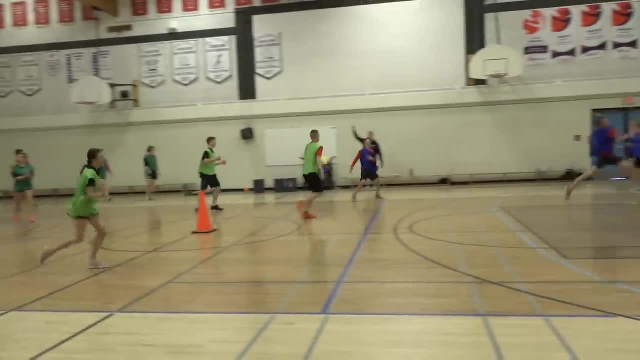 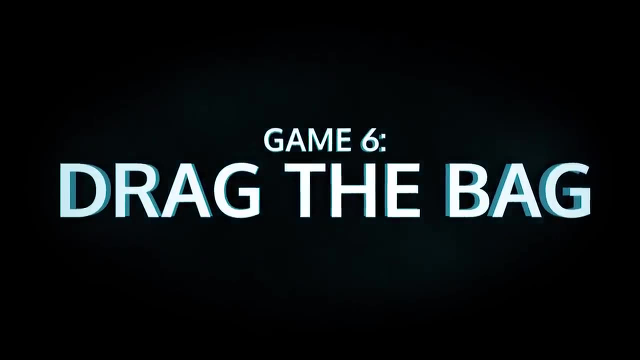 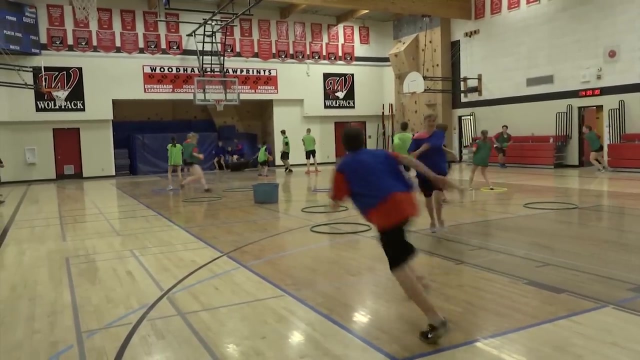 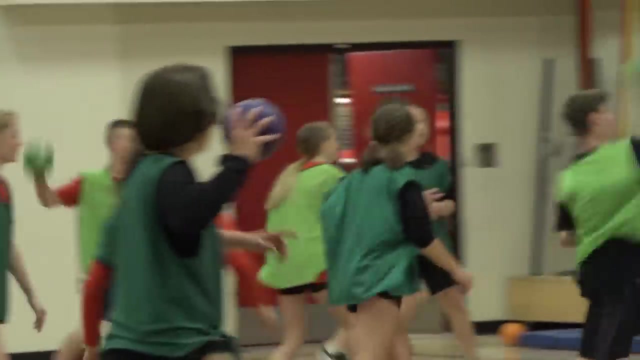 four points in one round. Oh, got him. The next game we're going to show you is called Drag the Bag. We play this game with our grade five to nine classes. however, this game can be modified and played probably all the way up to grade 12.. For this game, you will need a minimum of 20 kids and can also. 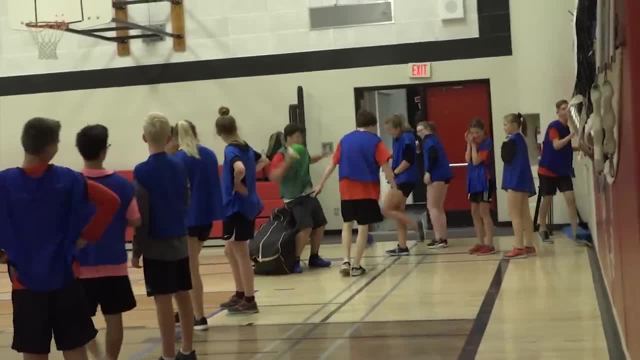 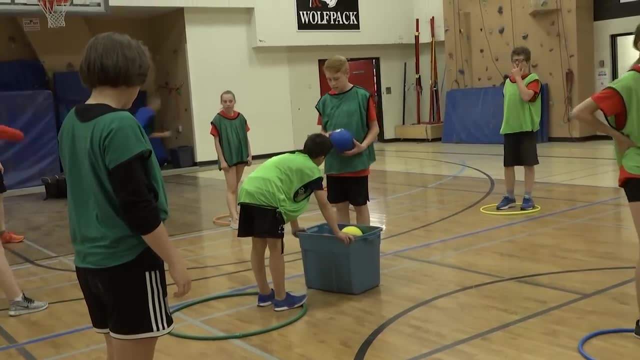 have a maximum up to about 60 or 70 kids, as you can make three teams and one team can sit off and you can rotate back on. The equipment needed are dodge balls, hula hoops and a bag full of heavy equipment We decided to use.